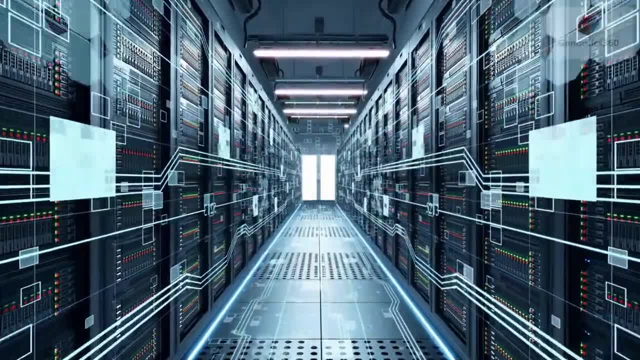 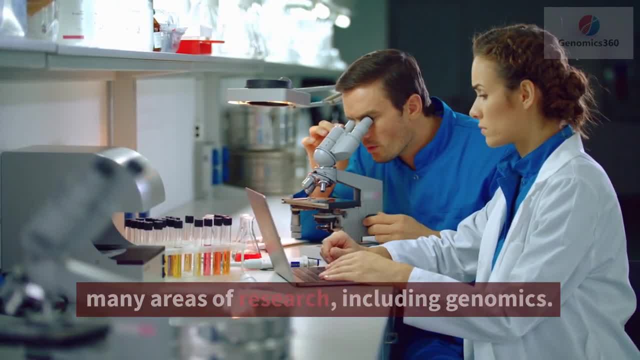 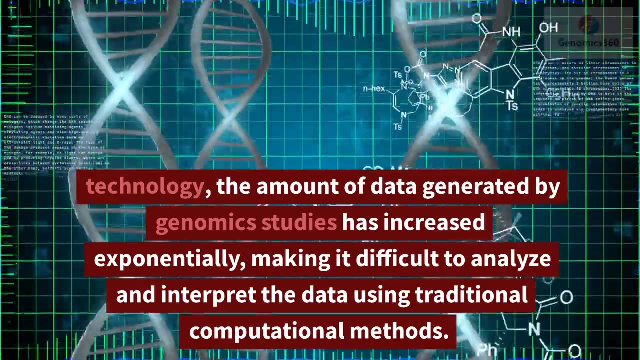 High Performance Computing for Genomics. High Performance Computing is a rapidly growing field that has revolutionized many areas of research, including genomics. With the rapid advances in DNA sequencing technology, the amount of data generated by genomic studies has increased exponentially, making it difficult to analyze and interpret. 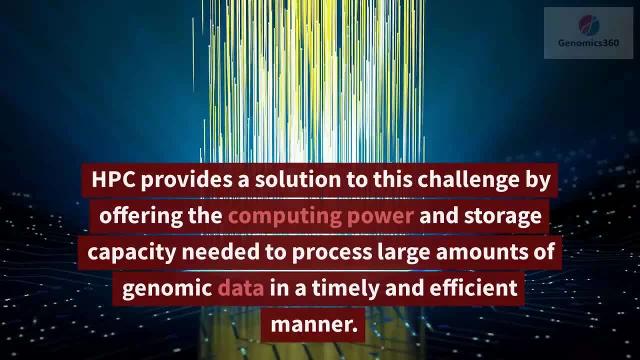 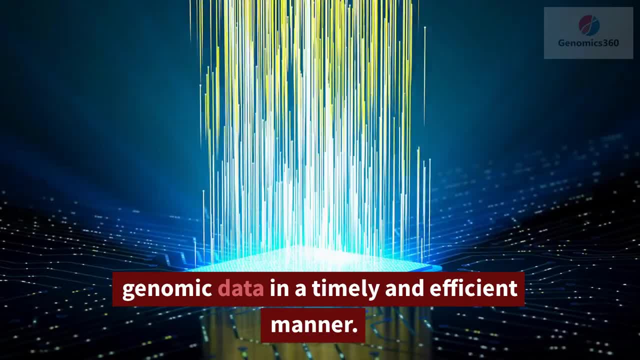 the data using traditional computational methods. HPC provides a solution to this challenge by offering the computing power and storage capacity needed to process large amounts of genomic data in a timely and efficient manner. In genomics, HPC is used for a variety of tasks. 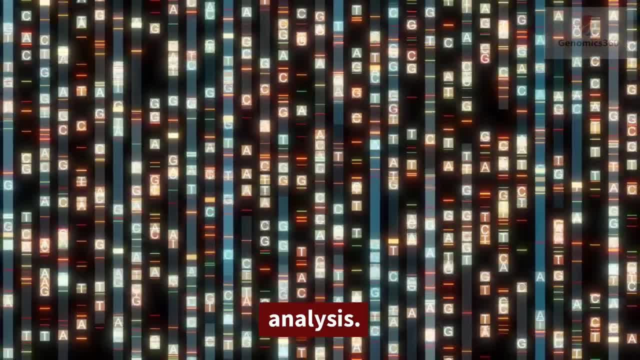 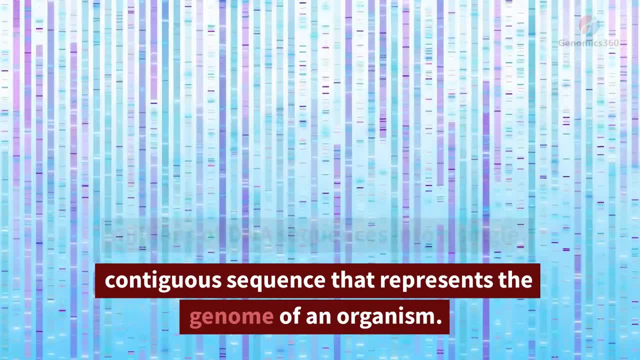 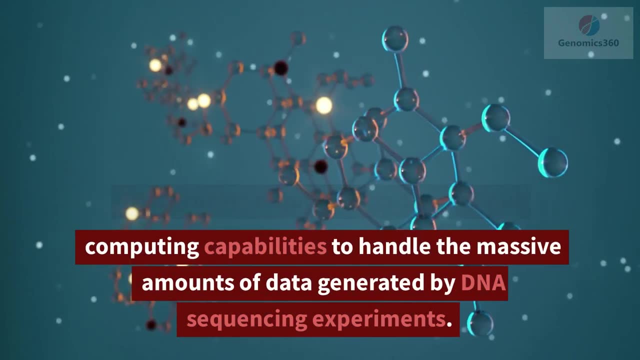 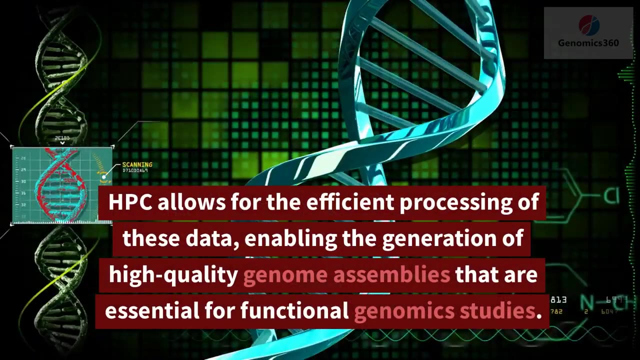 including genome assembly, gene expression analysis and genetic variant analysis. Genome assembly involves combining millions of DNA sequences into a single contiguous sequence that represents the genome of an organism. This process requires high throughput computing capabilities to handle the massive amounts of data generated by DNA sequencing experiments. HPC allows for the efficient processing of these. 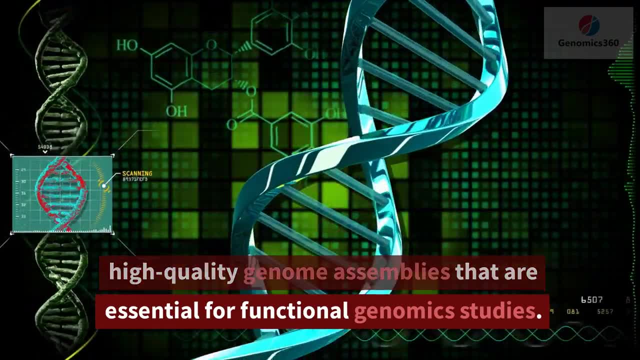 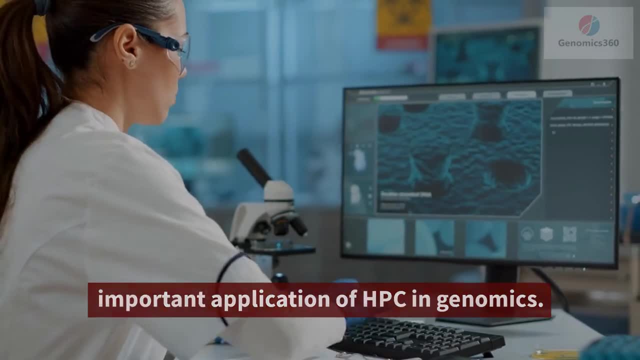 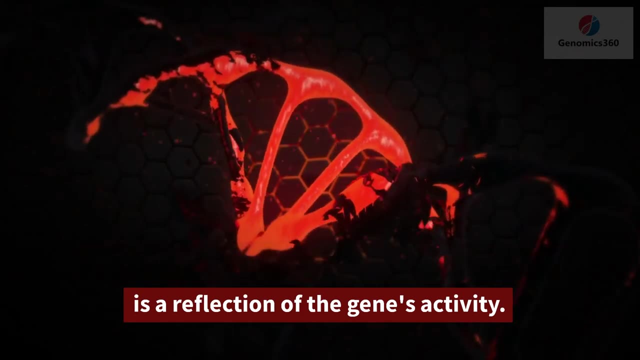 data enabling the generation of high-quality genome assemblies that are essential for functional genomic studies. Gene expression analysis is another important application of HPC in genomics. This type of analysis involves measuring the amount of mRNA produced by a gene, which is a reflection of the gene's activity. 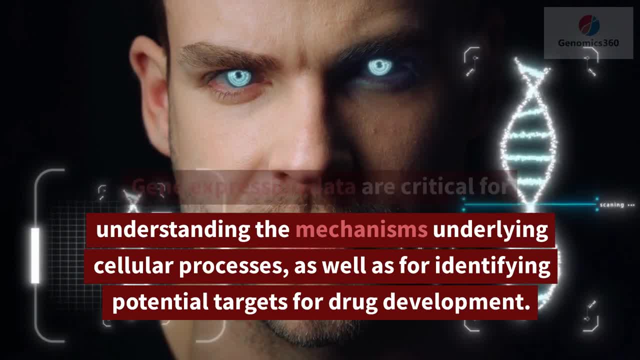 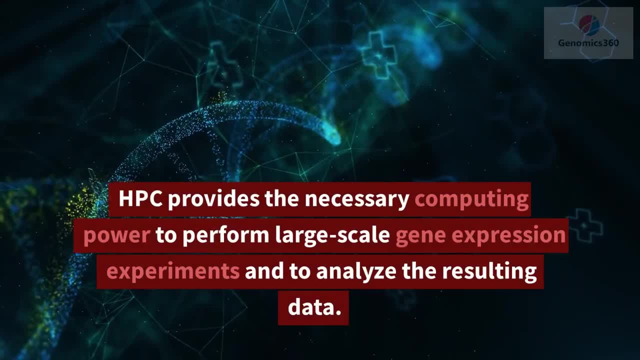 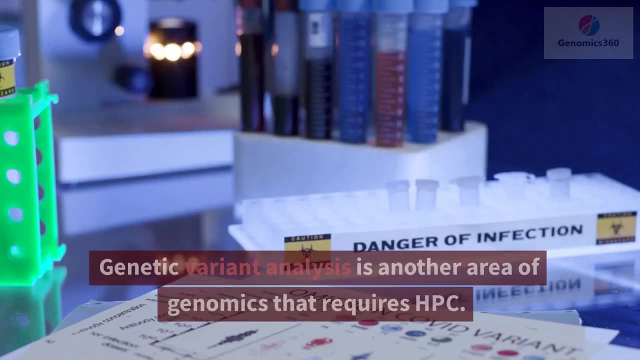 Gene expression data are critical for understanding the mechanisms, cellular processes, as well as for identifying potential targets for drug development. HPC provides the necessary computing power to perform large-scale gene expression experiments and to analyze the resulting data. Genetic variant analysis is another area of genomics. 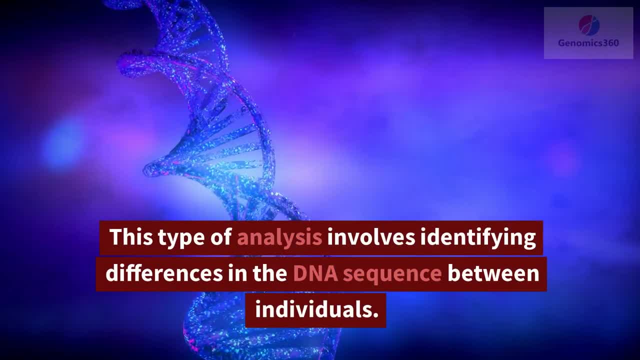 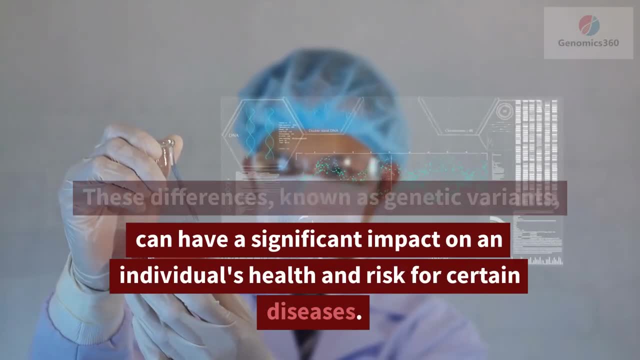 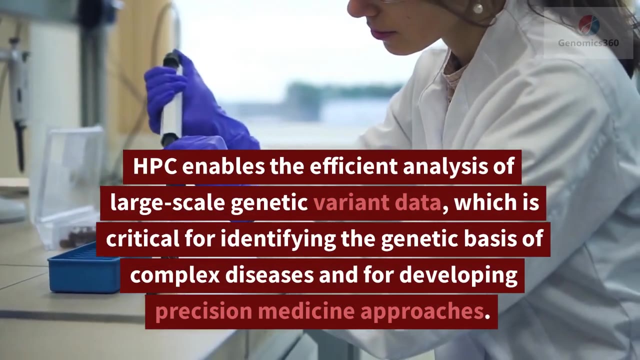 that requires HPC. This type of analysis involves identifying differences in the DNA sequence between individuals. These differences, known as genetic variants, can have a significant impact on an individual's health and risk for certain diseases. HPC enables the efficient analysis of large-scale genetic variant data, which is critical for identifying the genetic basis. 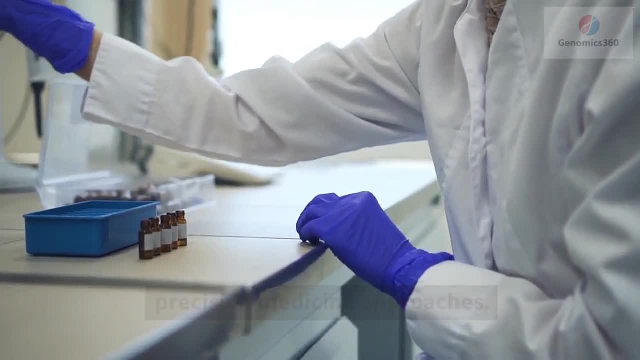 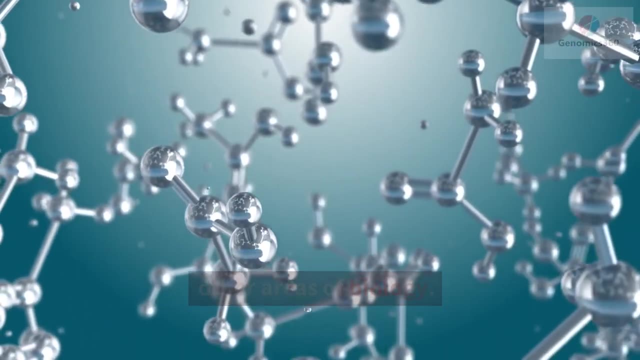 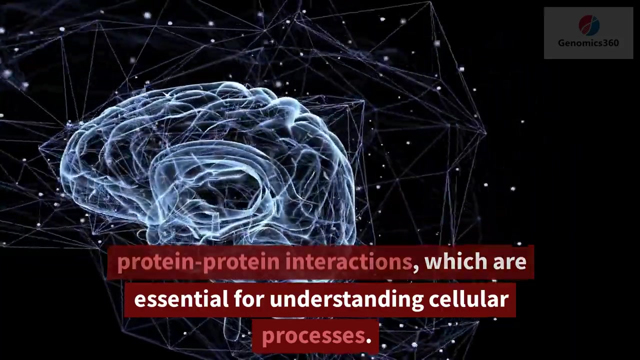 of complex diseases and for developing precision medicine approaches. In addition to its applications in genomics, HPC also has the potential to revolutionize other areas of biology. For example, HPC can be used to model complex biological systems such as protein-protein.